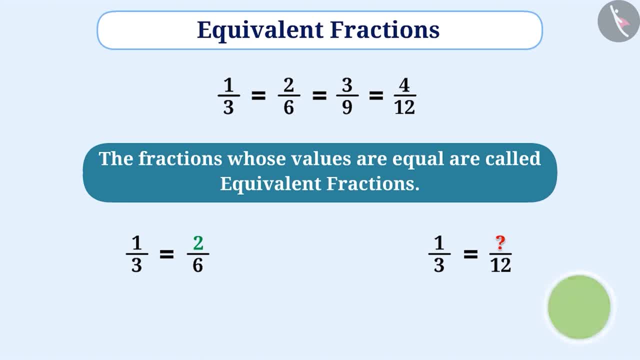 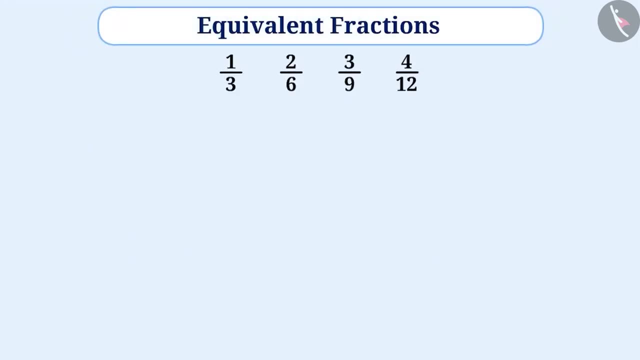 Think for a while. Absolutely correct. One third is equal to four twelfths. Now let's try to represent these fractions on the number line. If you look at these fractions then they may appear different to you, But if we represent them on the number line, that is, we are representing one-third, like. 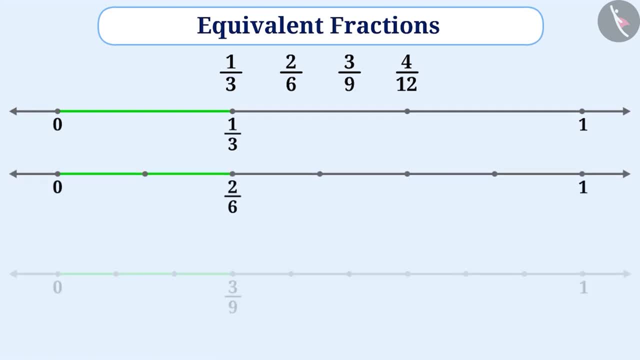 this, two-sixth like this, three-ninth like this and four-twelfth like this. then we can observe that all these fractions are marked at a similar point on the number line. Similarly, we can understand that the value of all these fractions is equal. 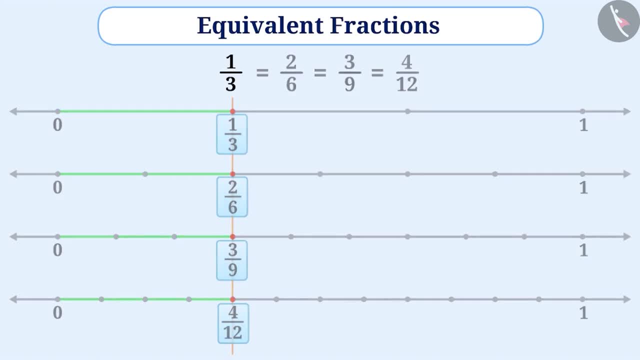 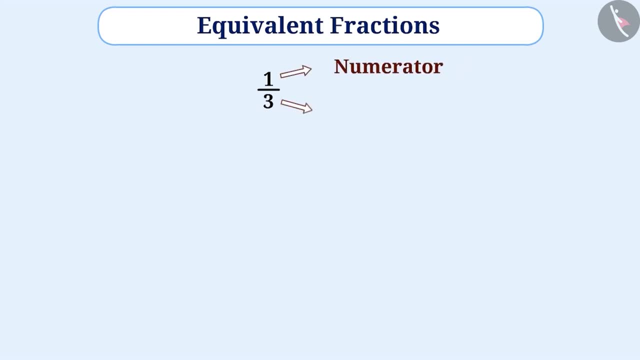 That means all these fractions are equivalent fractions. One of the ways to find the equivalent fractions of any given fraction is to multiply its numerator and denominator by the same number. For example, multiplying the numerator and denominator of one by three with two will give two by six. 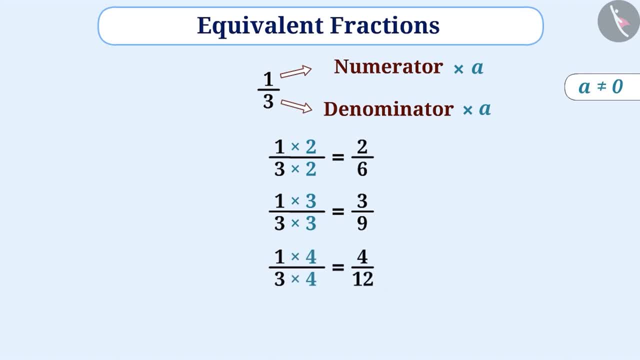 Multiplying with three gives three by nine And with four, three by nine And with four gives four by twelve, which are equivalent fractions. Similarly, in order to find the equivalent fractions of any given fraction, we can divide its numerator and denominator by the same number. 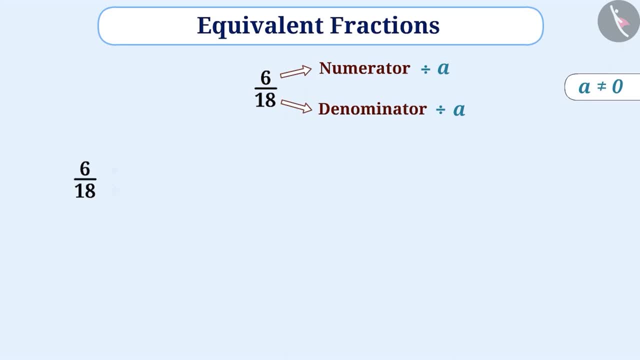 For example, to find the equivalent fractions of six by eighteen, the numerator and denominator can be divided by two, which gives equivalent fraction three by nine. Similarly, dividing by three will give an equivalent fraction of two by six. and similarly, dividing by six will give an equivalent fraction of one by three. 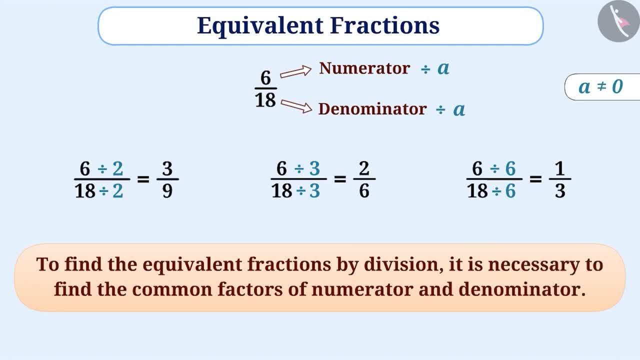 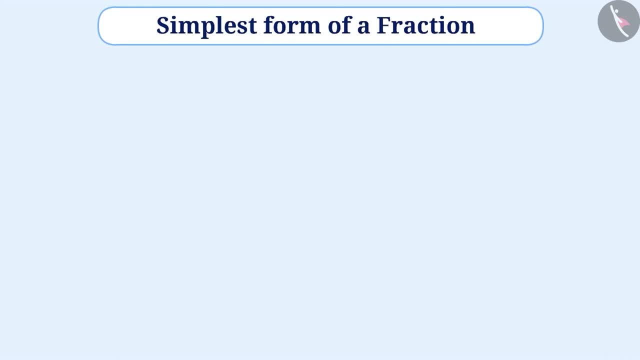 To find the equivalent fraction by division, it is necessary to find the common factors of numerator and denominator. Now let's understand what is the simplest form of a fraction. Suppose there is a cake and we have to divide it into twelve equal parts. 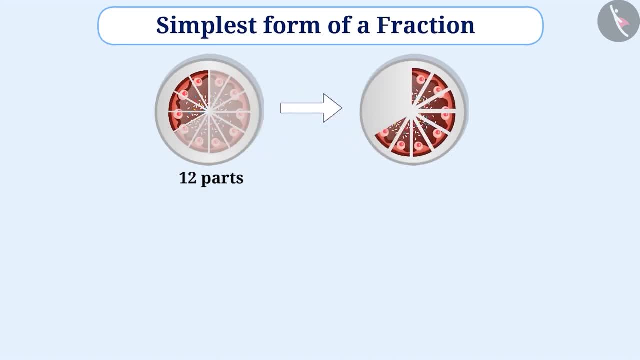 If we take out eight parts from it, then the fraction represented by the parts taken is written as eight by twelve. Here we have a cake. Here the numerator is eight and the denominator twelve. Since both numbers are even, therefore two is the common factor of these two numbers.